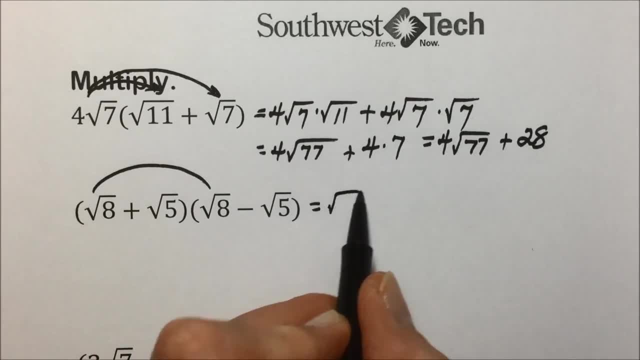 this, Multiplying the first two terms together, leaves us with square root of eight times square root of eight Outside terms. a positive times a negative is a negative. square root of eight times the square root of five Inside terms multiplied together, we have a positive times a positive is a positive. so we have a square root of. 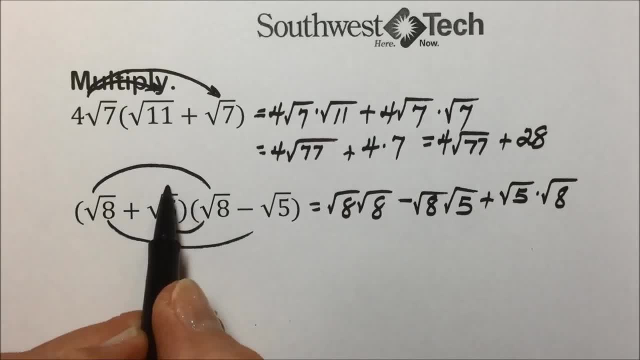 five times the square root of eight. And last terms: multiplied together, positive times, a negative is a negative square root of five times square root of five. Simplifying, we have square root of eight times square root of eight, that's square root of eight squared. 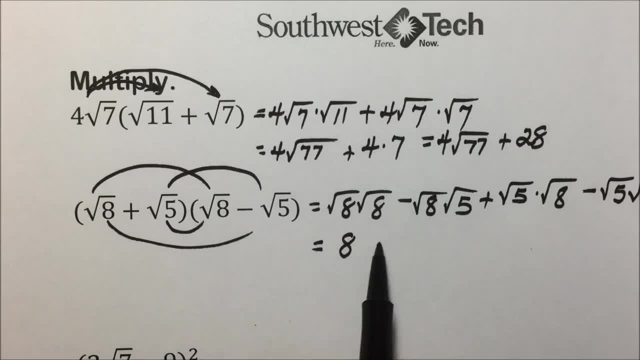 which is eight, We have next, multiplying these radicals together, a negative square root of forty. when we combine that product of radicals similar to the next one, plus square root of five times square root of eight, combined underneath one radical is giving. 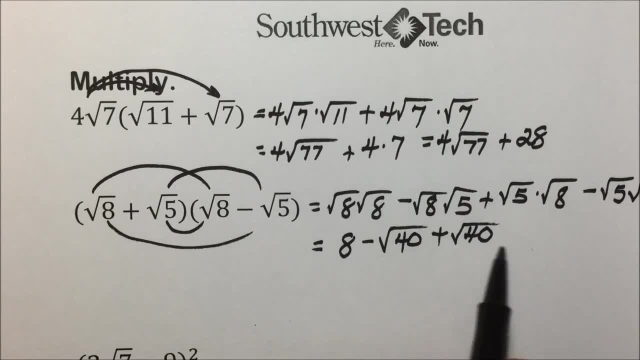 us the square root of five times eight or forty And the last term square root of five times square root of five, is the square root of five plus the square root of裸 times square root of nine times the square root of five, or exhibiting goods, And so the final. 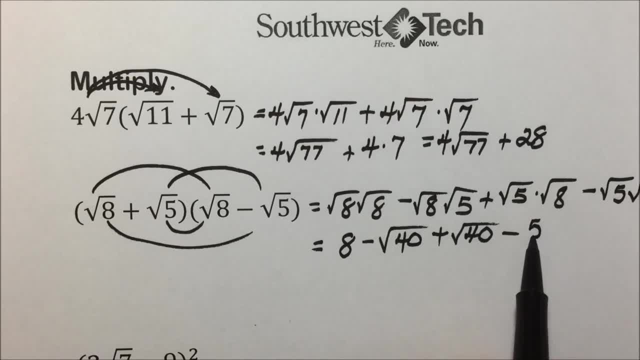 answer to this is counter約. Once again, there's no 느낌 and we use a skip- corrugation squared, which is 5.. Simplifying further, the radicals are similar or like radicals because of them both being square root and having a radicand of 40. 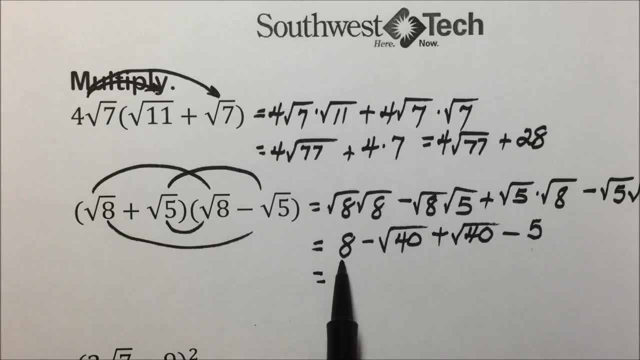 but a minus 1 plus 1. they're canceling out, leaving us with 8 minus 5 for a final answer of 3 for that answer. Interesting to note and something that we'll use very soon is that notice we started out with binomials that had. 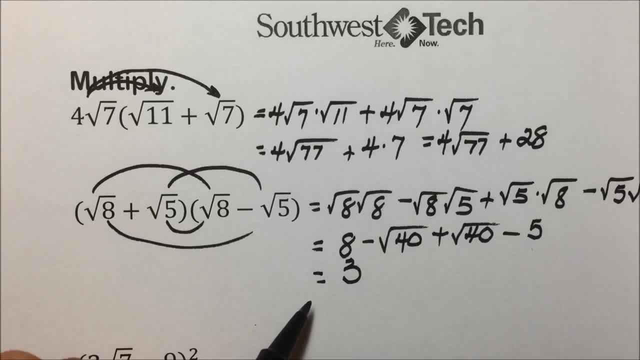 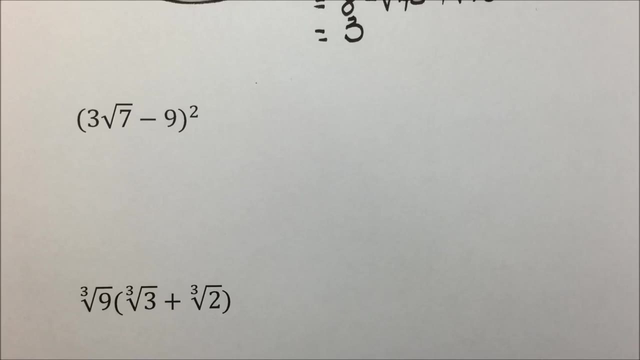 radicals in them, but our final answer was: radical free, something that we will use when we're rationalizing denominators or numerators with two terms. In this next problem, they're asking us to take this radical expression and square which first. we'll rewrite this. 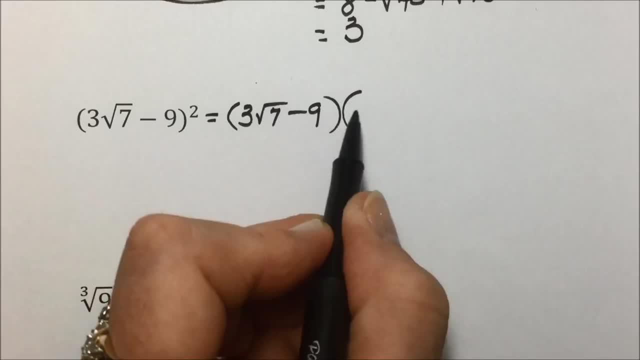 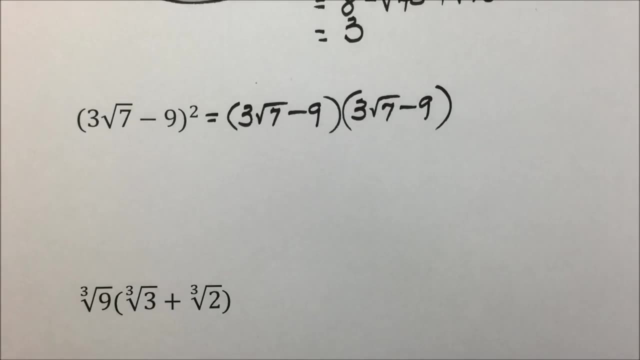 and we're going to use the same problem, but we're going to use the same as an equivalence of 3 times the square root of 7 minus 9 times itself, and then use the FOIL method, similar to what we did in the last problem. 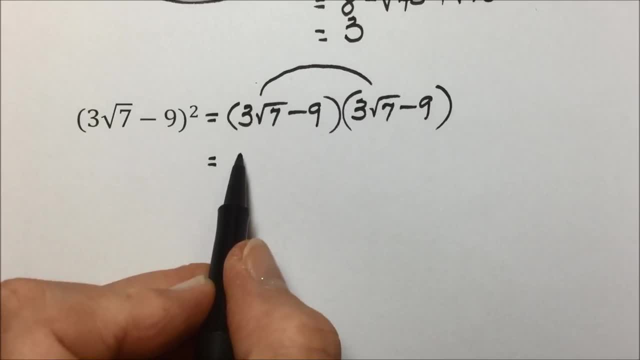 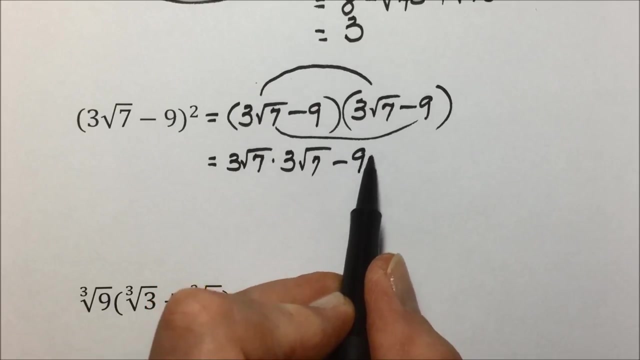 First terms: multiply together gives us a 3 times square root of 7 times 3 times the square root of 7.. All side terms multiply together: a negative times a positive would be a negative 9 times 3 times the square root of 7.. 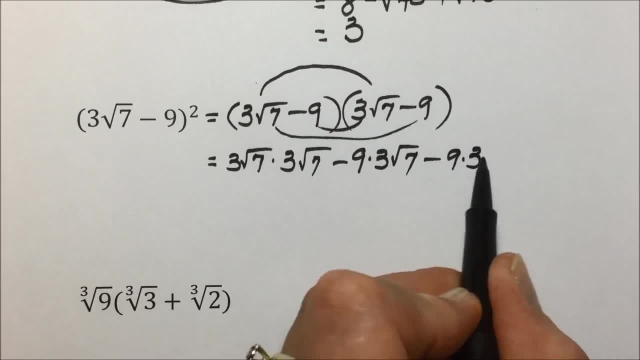 Inside terms, we end up with the same negative 9 times 3 times the square root of 7.. And last terms: a negative 9 times a negative 9 is a positive 81.. Now you could have simplified as we went, but just to demonstrate what's happening with the multiplication. 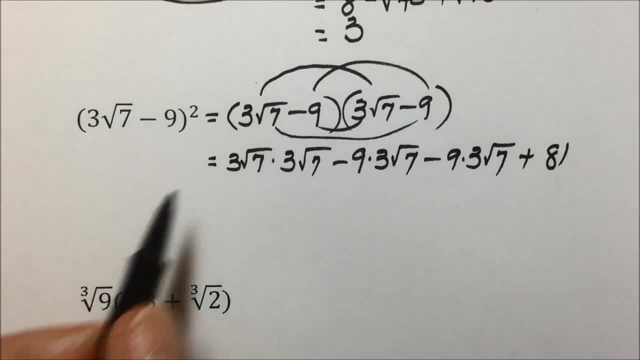 so that you see, To see the simplification, we have integers multiplied together. that would be a 3 times 3, and if we rearrange this using commutative property, we have square root of 7 times square root of 7,. 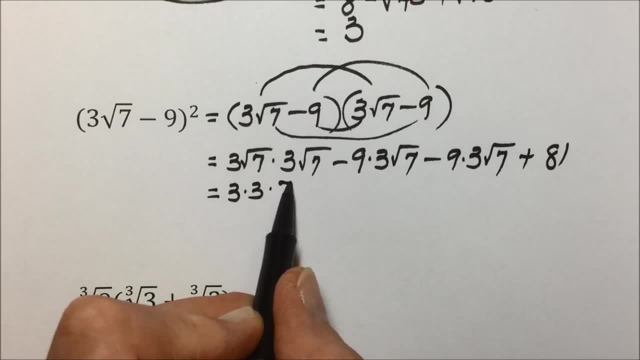 which is square root of 7, squared or square root of 49,, which is a 7.. In the next term, we have the integers out in front that we can multiply: 9 times 3 is 27,, square root of 7,. likewise, same with this: 9 times 3 is 27,, square root of 7, and our 81 on the tail end. 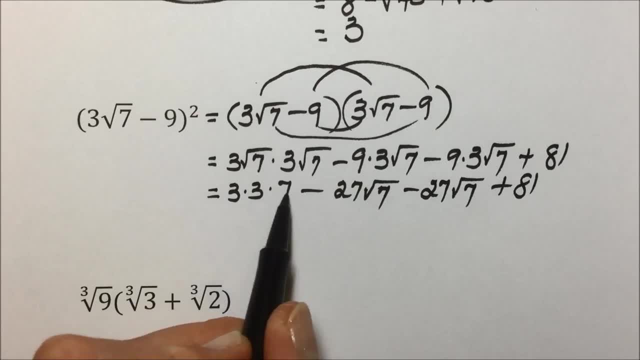 Multiplying here on the first term, we have: 3 times 3 is 9, times 7 is 63.. These are similar terms. a negative 27 plus a negative 27 is a negative 54, square root of 7,. 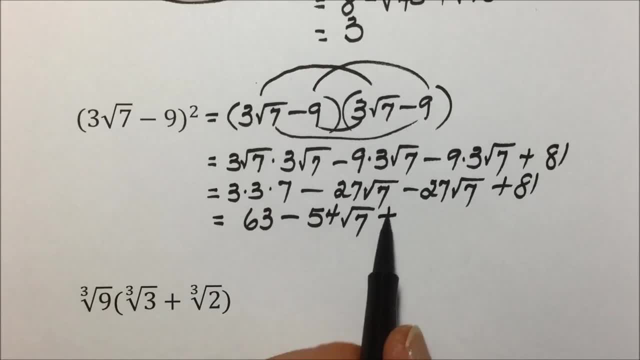 because of these being like radicals, Plus the 81,. and our final step, then, can we simplify further? We have integers that we can combine, which we end up with adding these together: 144 minus 54 times the square root of 7.. 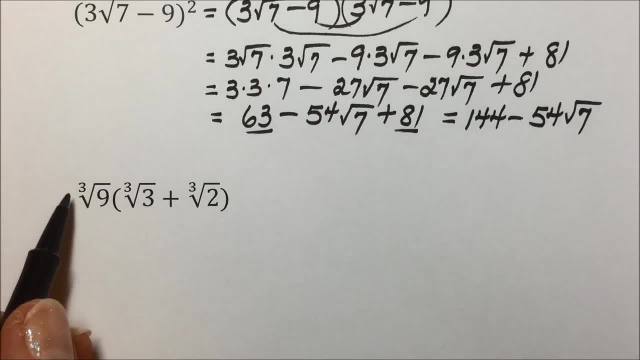 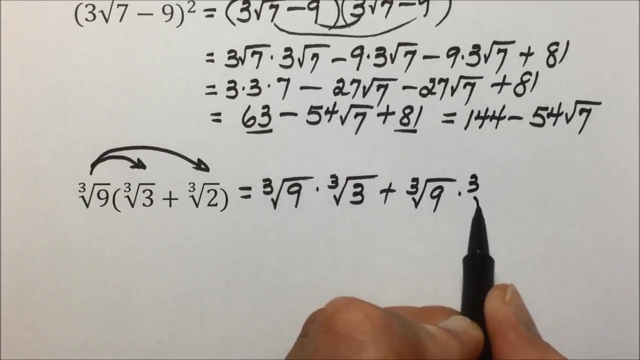 In this last example we have essentially- you can think of this- as a monomial times a binomial. We'll use the distributive property to eliminate the parentheses And that will result in the cube root of 9, times the cube root of 3, plus the cube root of 9, times the cube root of 2..